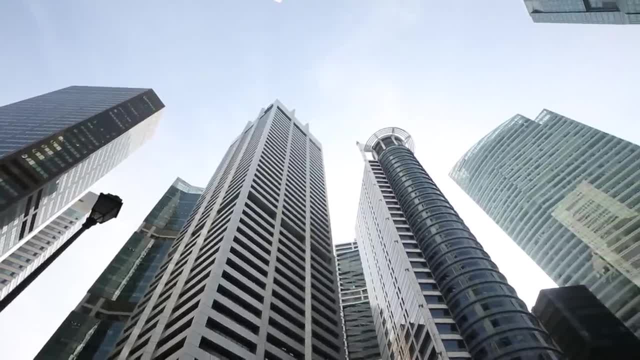 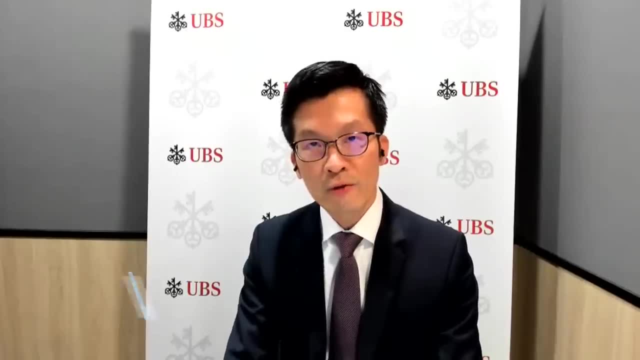 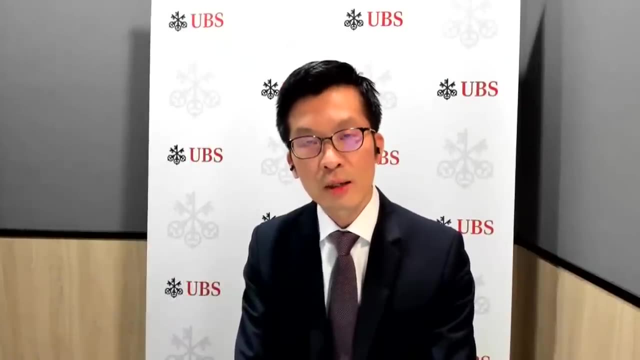 But this does not mean that it wants the SING dollar to depreciate. In fact, its policy is for the SING to have a gradual and modest appreciation. Keep in mind that inflation in Singapore is still likely to be a bit sticky, So for that reason the MAS is still likely to keep SING on a strengthening path. 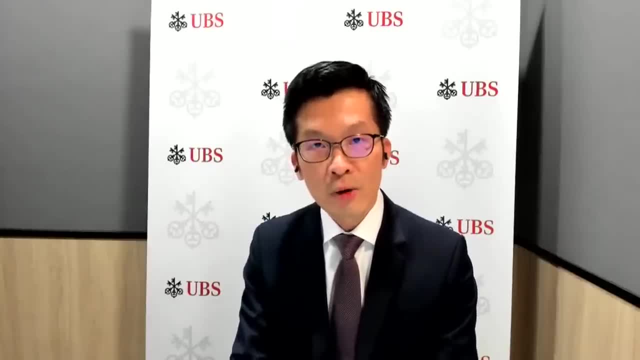 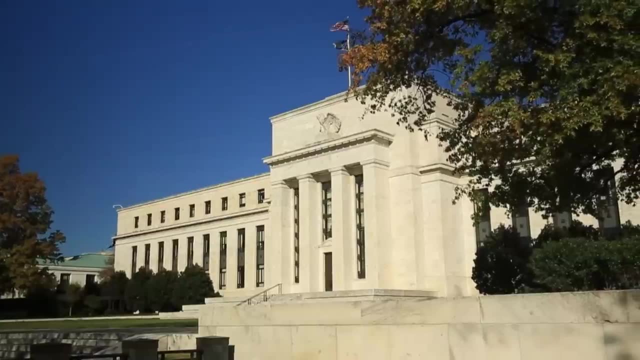 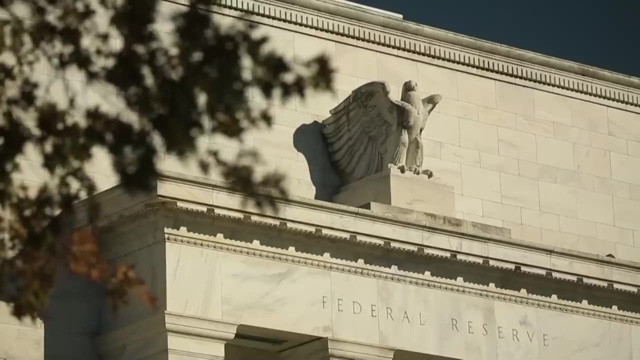 But it is just that, because global growth is also decelerating and the MAS would be mindful not to strengthen the SING in an excessive manner. The big mover in the currency markets this year will be the impending monetary easing by the US Federal Reserve. That should give a boost to all Asian currencies. 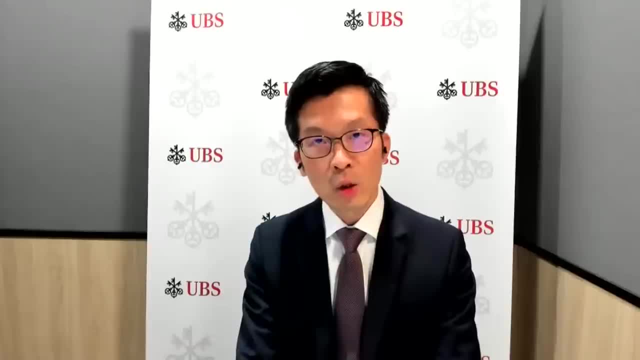 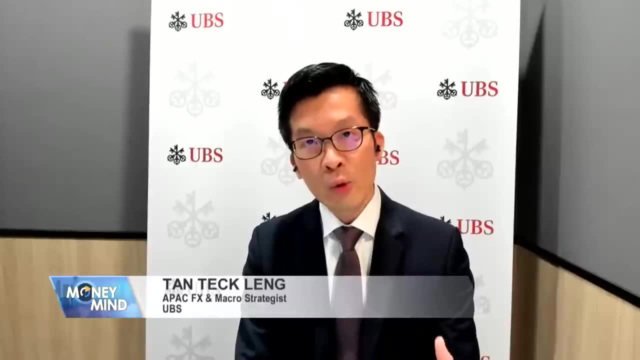 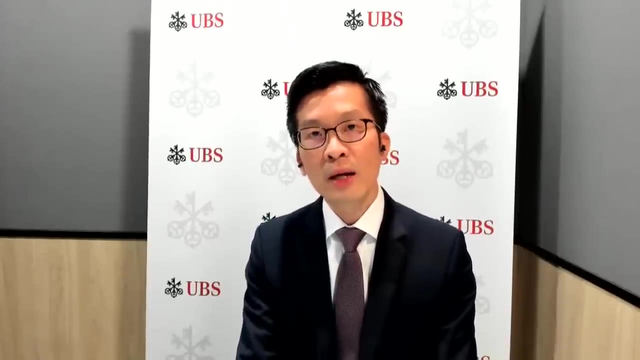 There should be, theoretically speaking, no losers. It is just who will win more and who would win less. So, for the relative winners within the region, we would say the Japanese yen would be one of the biggest winners, simply because, if you recall, back in 2022, the Japanese yen was the biggest. 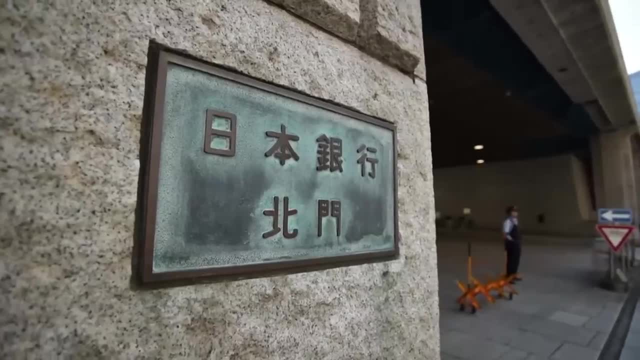 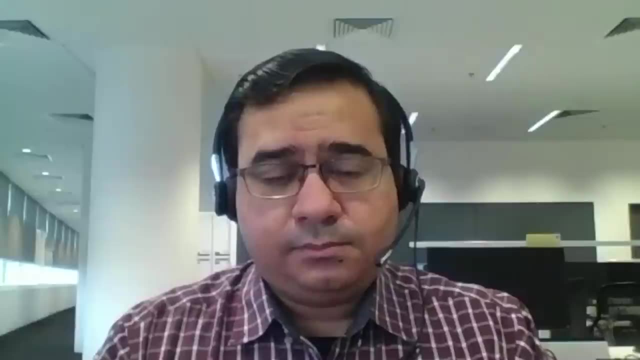 loser when the Fed was tightening, And that was because the Bank of Japan was actually keeping interest rate policy very tight, And that was because the Bank of Japan was actually keeping a record high For the cameos, the QM 어때. 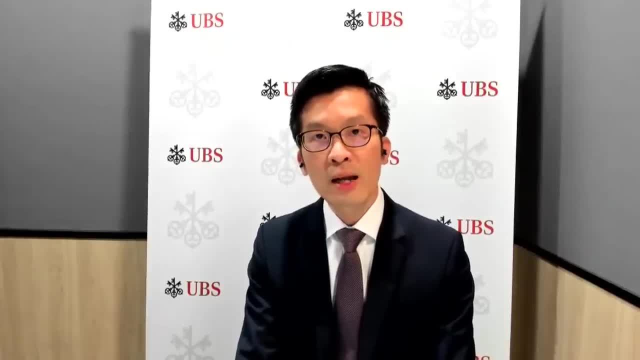 Veryقيım. I think also very accommodative, really comfortable. But I think, if we can add, it is not just about the Fed easing monetary policy for 2023, because 2023 is also about China reopening. So, on that factor as well, there are other big winners, in Asia, For example. the Australian dollar is said to benefit strongly from the commodity linkage with China and the Thai baht as well, with Chinese tourists returning back to Thailand. We are also looking at the time, but as a strong beneficiary, So with the rise of other currencies in the region. 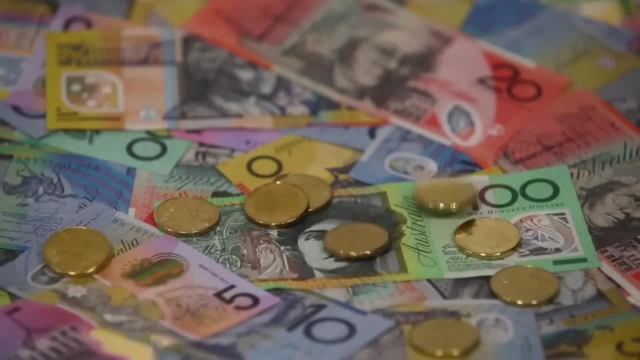 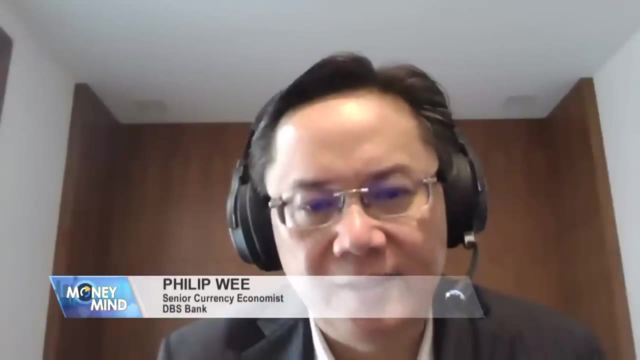 should investors turn away from the SING dollar? I'm not a seller of the dollar against the SING around these levels. Dollar SING has been in this $1.31, $1.46 range since the currency war in 2015,. and right now we are near the bottom. So the last two times dollar bounced from $1.32.. It rose to about $1.38 in 2018, $1.37 in 2021.. I have about $1.36 as my target for this quarter. When you talk about safe haven, you generally expect some unexpected shock. When I formed Outlook, I was looking for relative value and soft landing once the Fed and other central banks are done with their hikes. So I don't I think that the SING will be favoured.